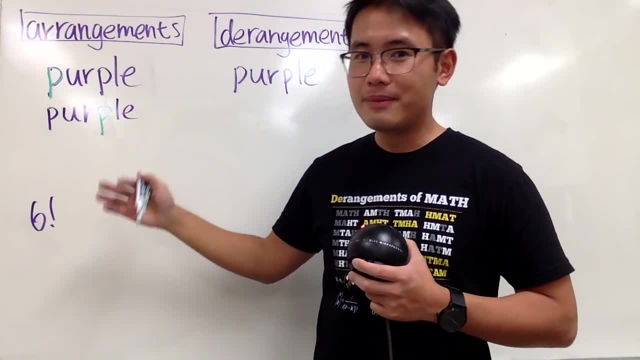 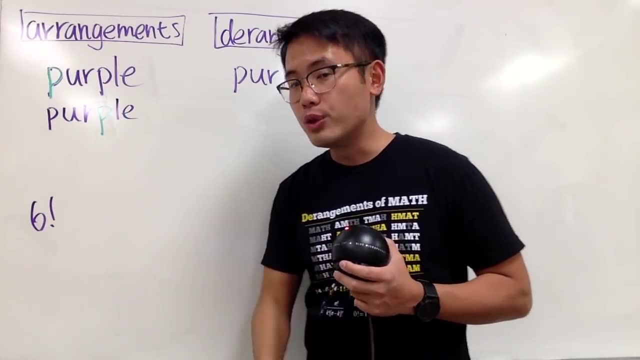 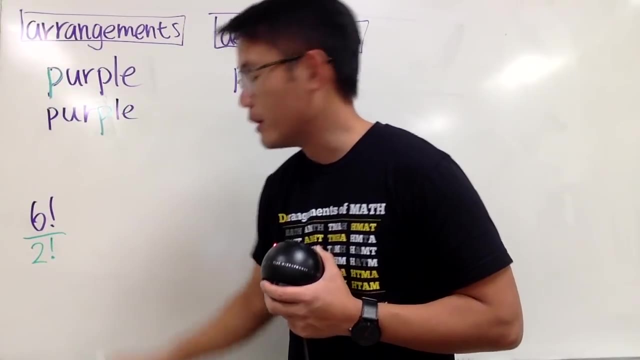 right here in green and then L E. Well, in this case, this is still purple. So you don't want this to happen. What you do is you will have to divide it by. We have two P's being the same, so you have to divide it by two. factorial. This is not. 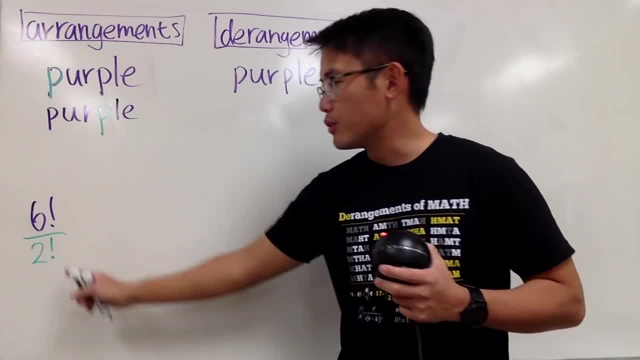 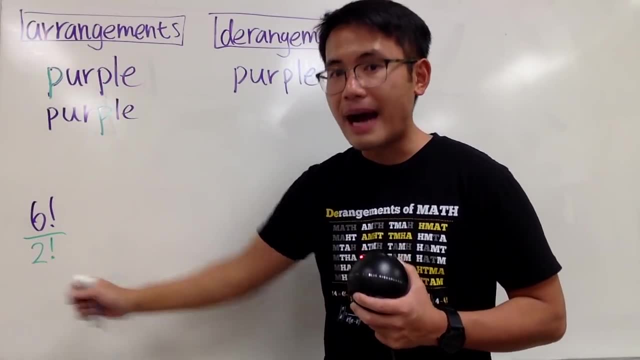 just a two, Even though two factorial is two, but you will have to divide it by two factorial. The idea is that imagine if you have three P's right here in this word, then you have to divide it by three factorial right, Because you have to think. 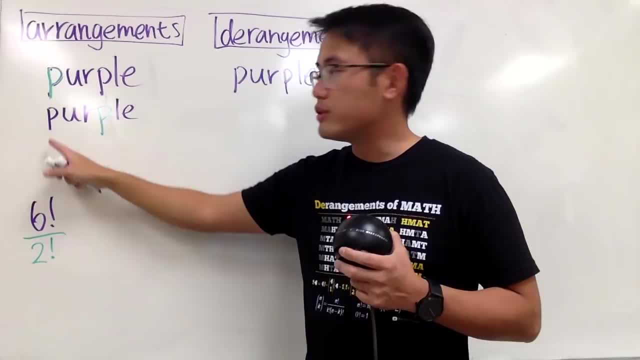 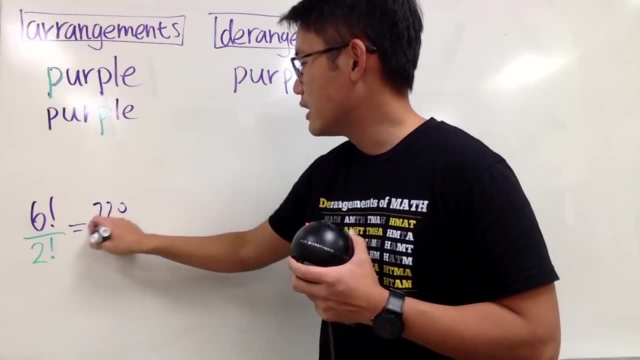 about how many ways to permute or to arrange this P and that P in these two spots. So this is pretty much it. Well, work this out on the top of 720, divide it by two, Two factorial, which is two, So altogether you get 360, like that, All right done. 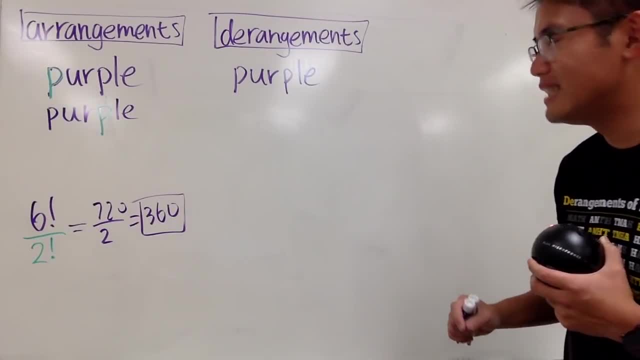 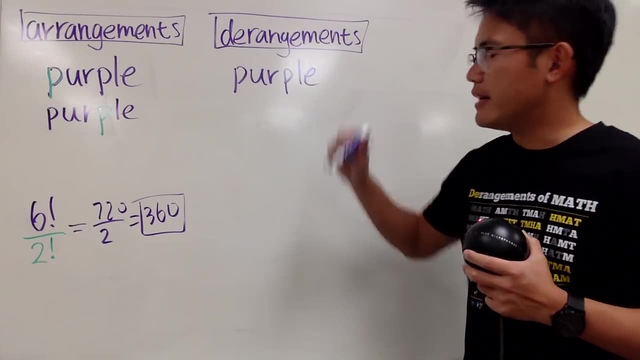 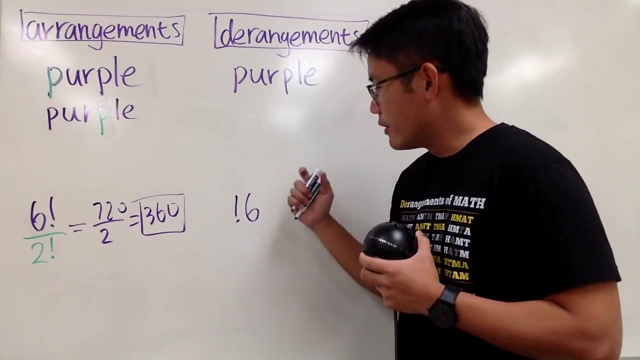 Now this right here is the main dish. That was just the little appetizer. Hmm, derangement with repetitions. I have six letters. Of course I should have sub factorial to help me out. sub factorial six: This is the usual number of 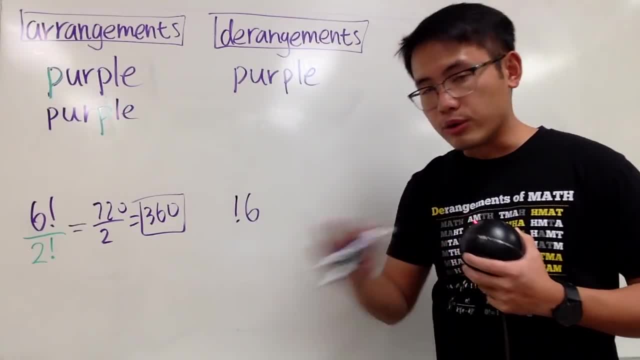 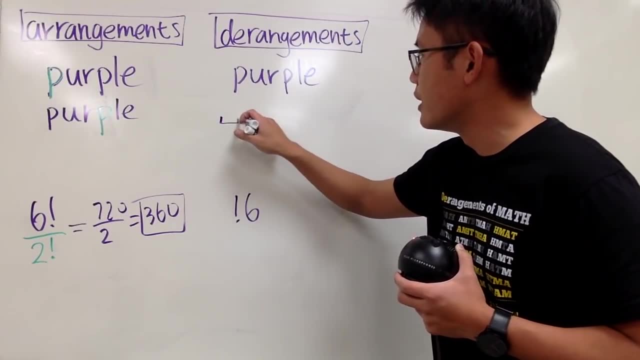 derangement When we have six letters, they are all different. But if I have this P and that P being the same, then we have to be really careful. And let me just show you guys, the first scenario right here. So suppose I am going. 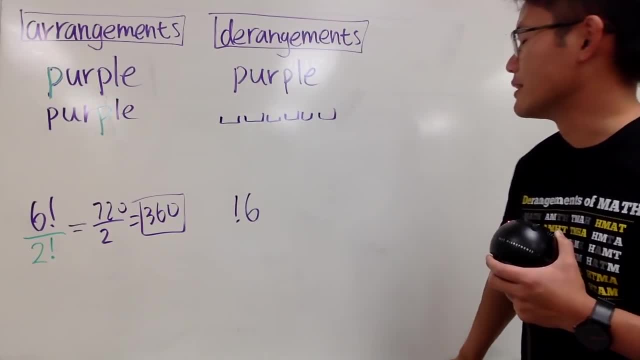 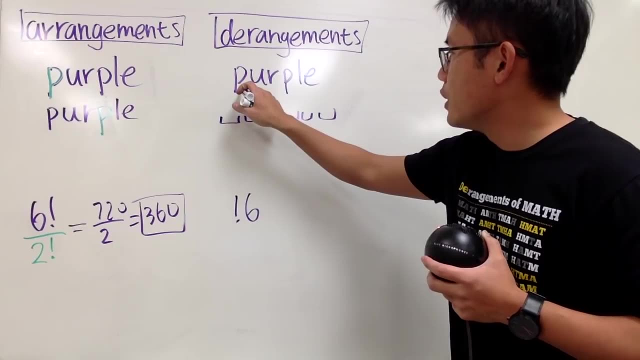 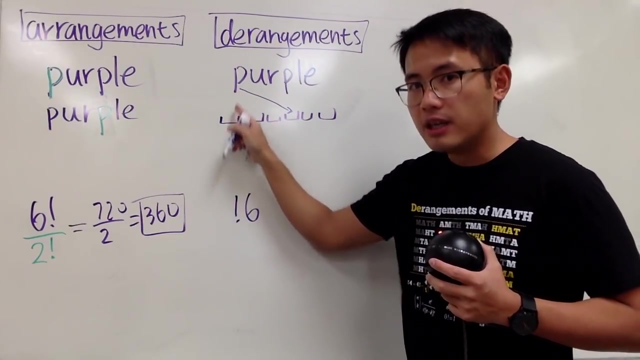 to draw the corresponding spots or the slots like this. Well, one of the issues is that, if you put this P right here, yes, you deranged this P because this P is not in the first place. So you did derange this P, But the problem is that the moment, 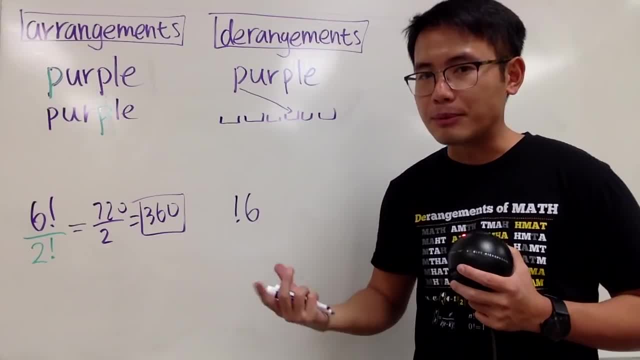 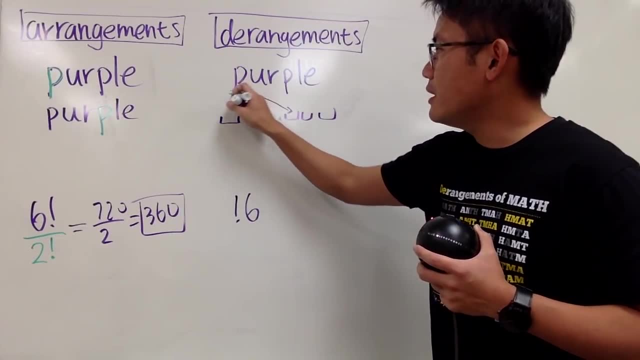 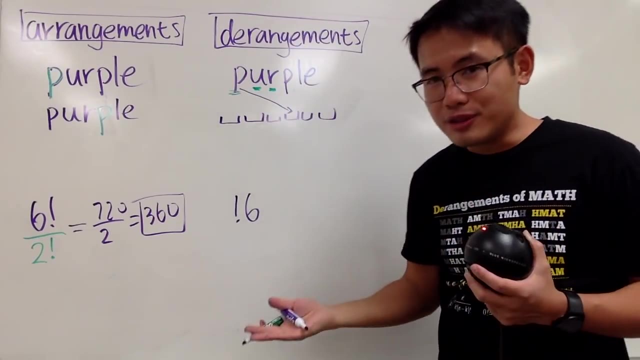 you put this P right here. that's a false derangement. We have to subtract that from the total of the sub factorial six. Well, we are deranging this P and then we are also deranging this P. you know what I mean. this U, this R and this P is not deranged because 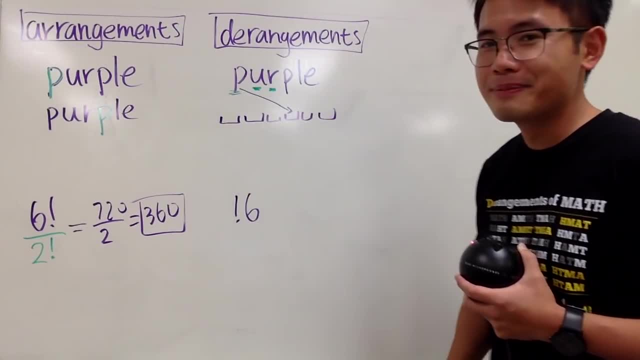 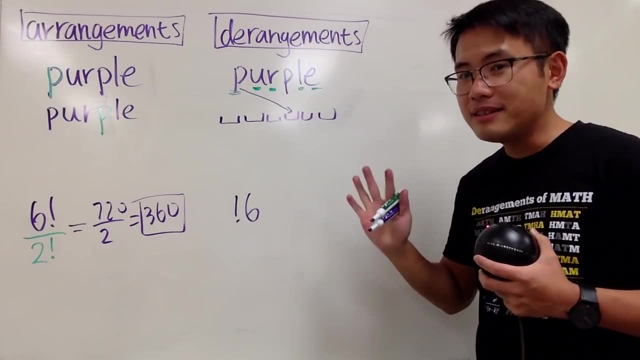 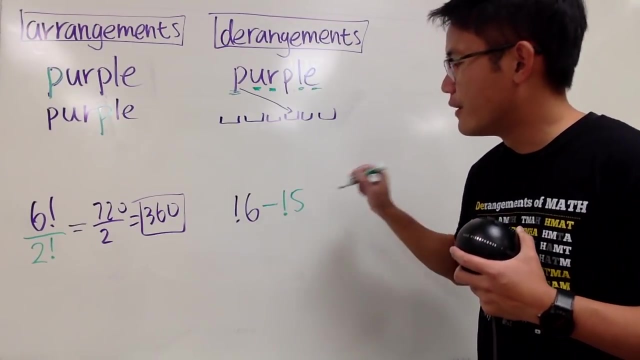 you always see the P right here thanks to that guy right. So in fact we are deranging this, this, this and this and that. So technically we have five things that were deranging and these 5 things are all different. So I will have to subtract sub factorial of 5.. 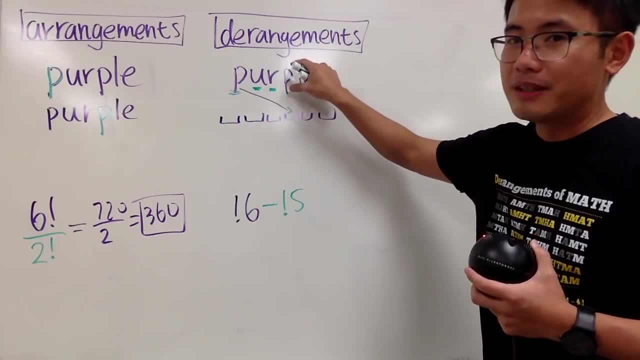 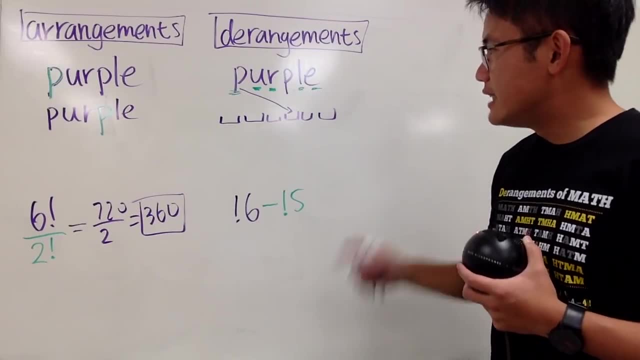 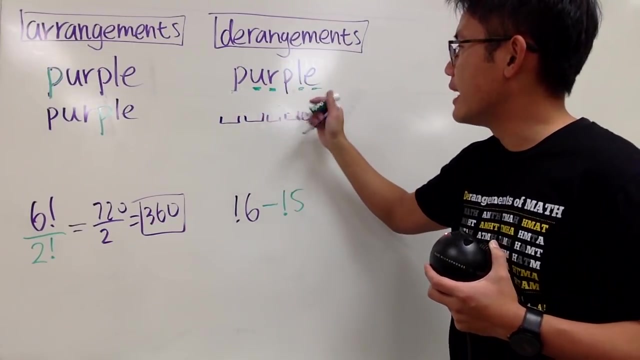 So that's the idea: Just ignore this p, because there's no hope, because you always have this p already. Technically you deranged this 5,, 6, right. Similarly if you deranged this p, but if you put this p right here instead. so I will put this down like this: 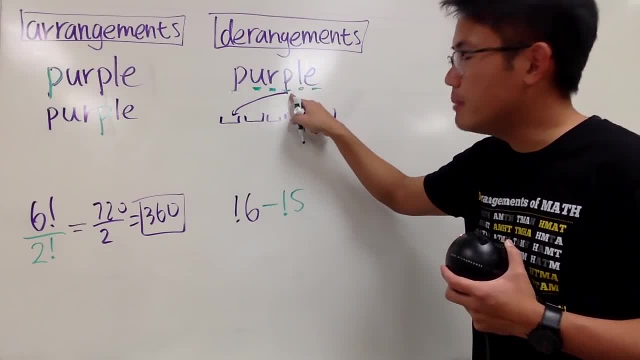 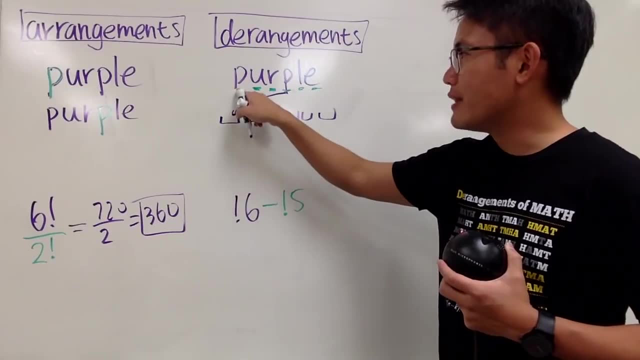 Okay, Well, yes, you deranged this p because this p is no longer here, but you always have a p in the first place, So you are not deranging this p, You are deranging this, this, this, this, that. 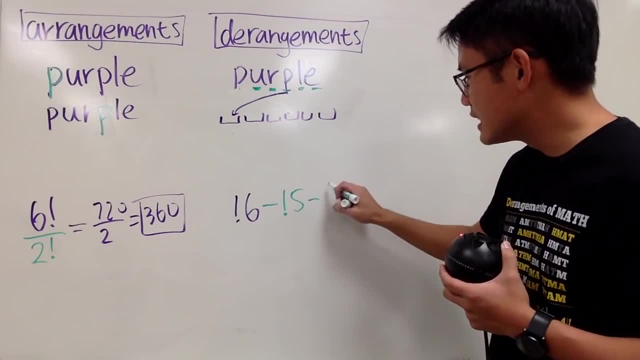 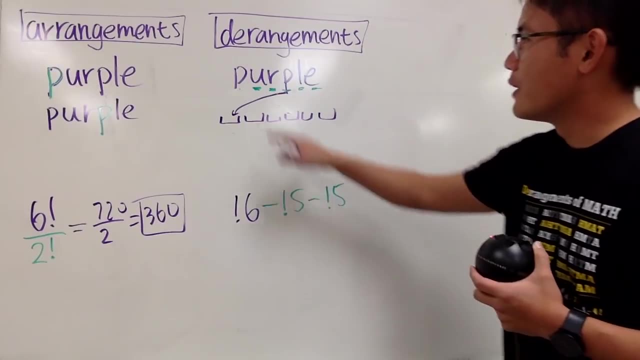 still sub factorial of 5.. So you have to minus sub factorial of 5.. Well, well, I know what you guys are thinking. What if we have the first p goes here and that p goes here? So let me just 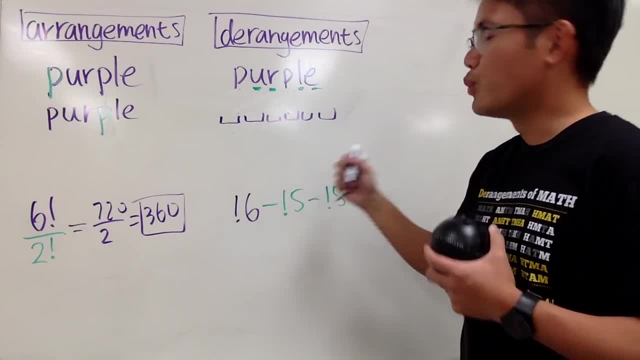 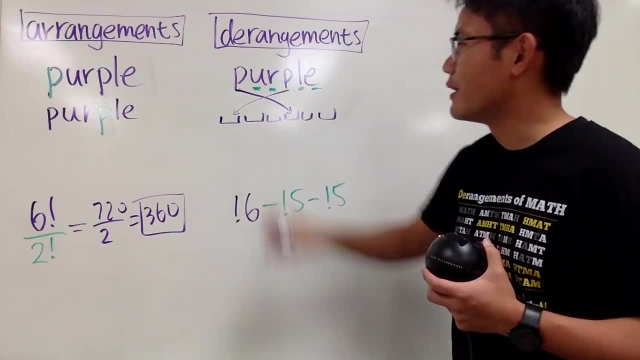 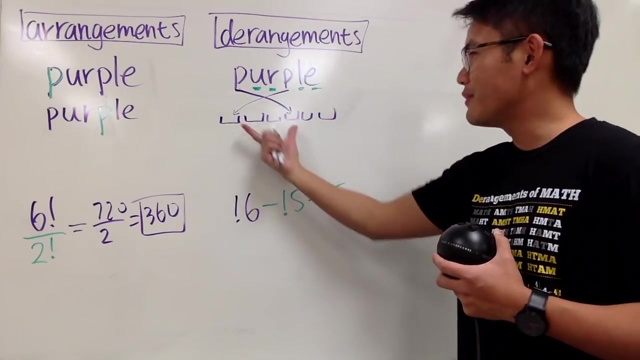 erase this. The last situation we'll have to worry about is this p might go here. That's bad. In the meantime, this p also goes there. In that case, you are not really deranging this p. Well, you are not really deranging these two p's, because you have these two p's right here in. 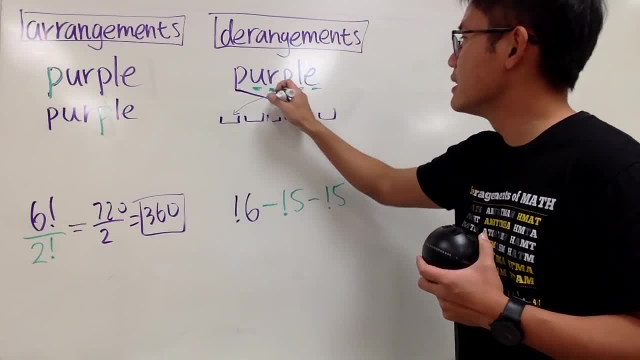 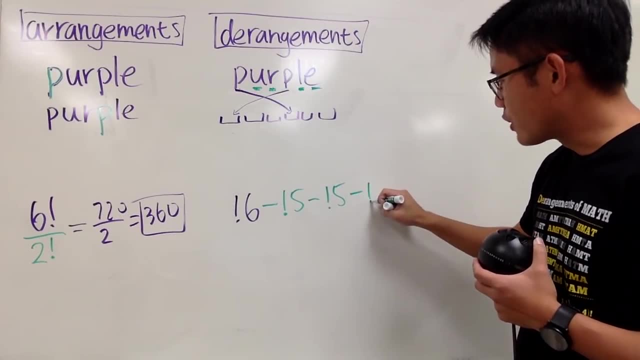 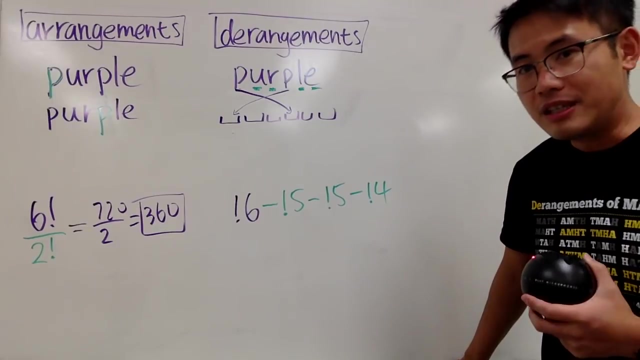 this spot. So what you're doing is just deranging this, this, this and that, So you have four things and they are all different. So you have to minus sub factorial of 4, well, this is really really nice, isn't it? So this is it, but you have to be careful. 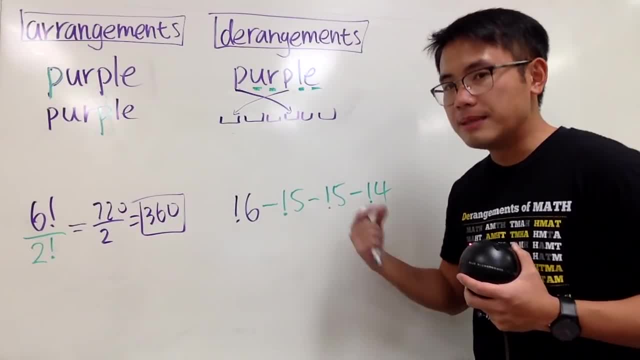 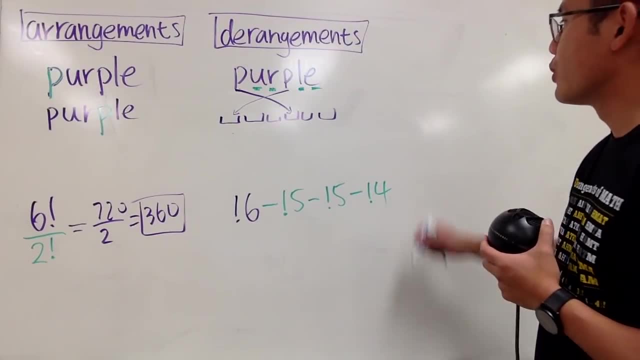 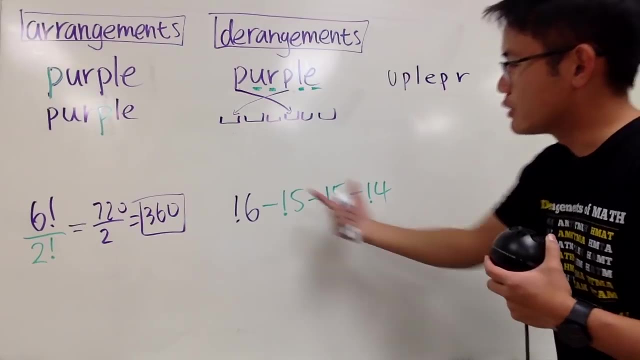 because similar situation, this right here seem to be true derangement, but we are double counting just like that. Why? Because let me just draw you guys a derangement right here. Suppose you have this is a derangement, right. But when you have a derangement which is right here already, 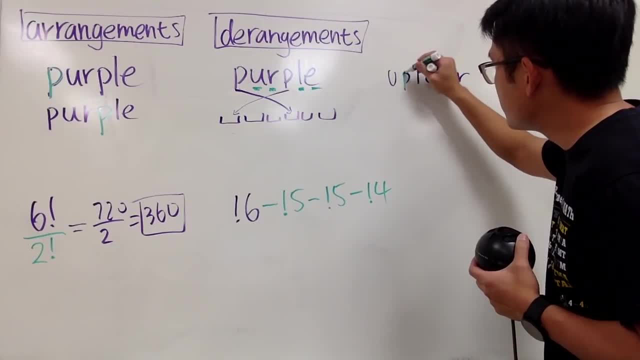 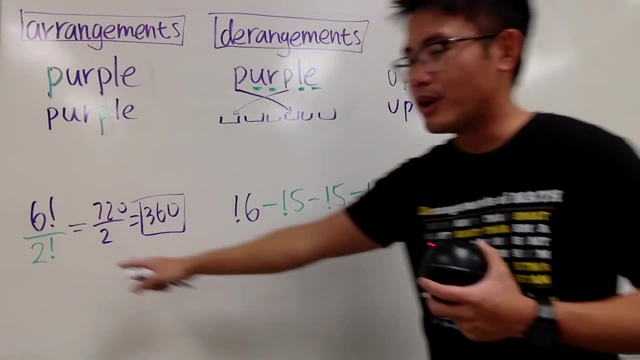 well, I will do the same trick. like that, I may have this p here and that p If you switch. well, you don't want this to happen. so what can we do? Yes, you got it. We are going to divide it by two: factorial, just like. 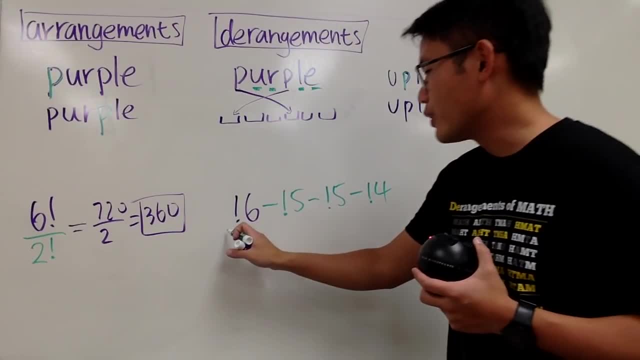 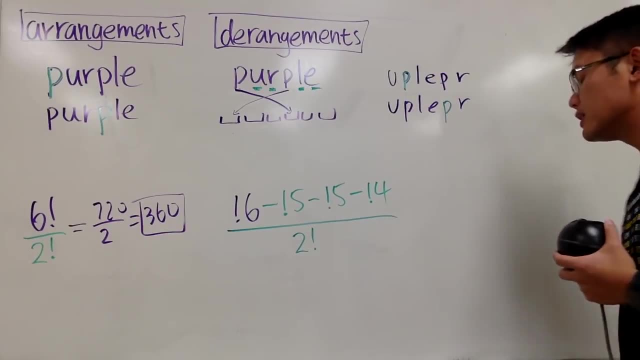 this as well. So, among this so-called derangement, we want to divide all the repetitions, so divide it by two factorials. So this is pretty much it. Now, the deal is that how do we calculate sub factorials? So I'll put this down real quick. Remember the list that we